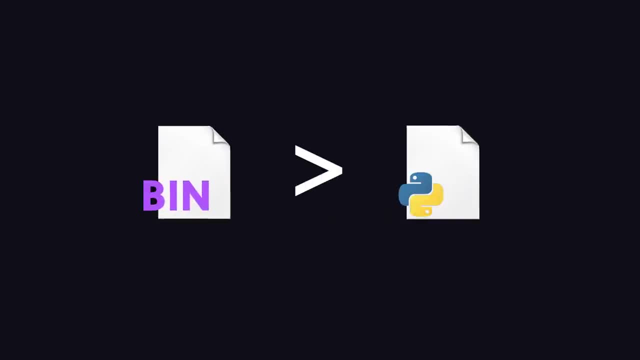 code is compiled down to machine code, which means it generally outperforms interpreted languages, But it's famous for its extremely fast compile times, made possible by innovations to dependency analysis, And even though it's a statically typed language, it performs type inference to deliver a syntax that is very concise and practical. It also has a package. 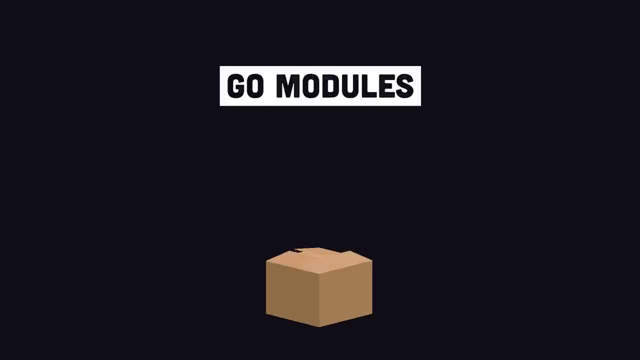 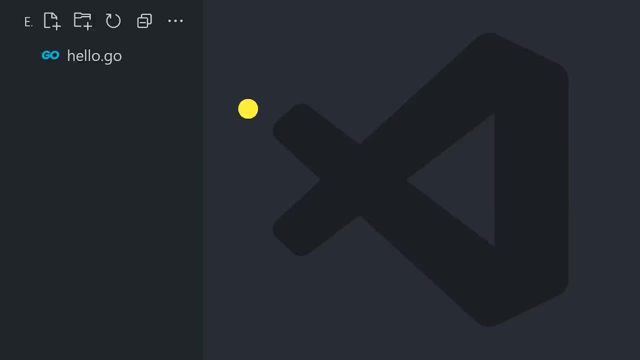 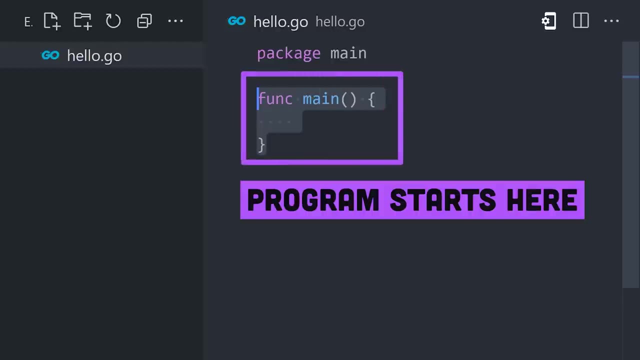 and module system, making it easy to import and export code between projects. To get started, install Go. Open an empty directory on your system. Create a file ending in go. Then add package main at the top to create a standalone executable. Then declare a main function, which is where: 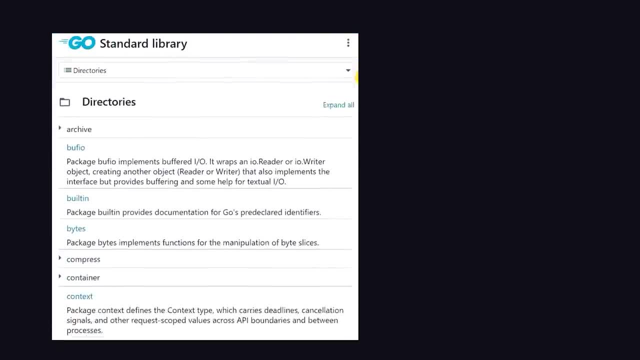 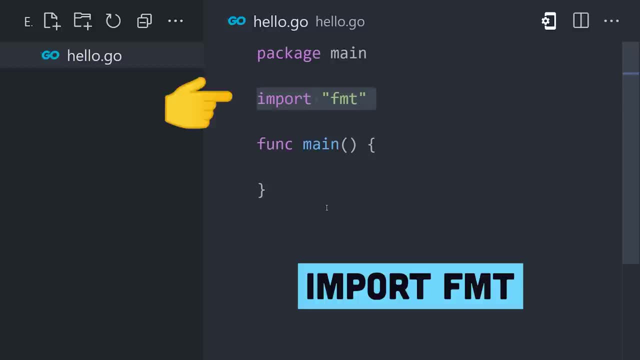 your program will start executing. Go has a standard library of core packages to handle common requirements like math, networking or formatted IO. By importing fmt we can print a line to the standard output, Then run the go build command and it quickly compiles. 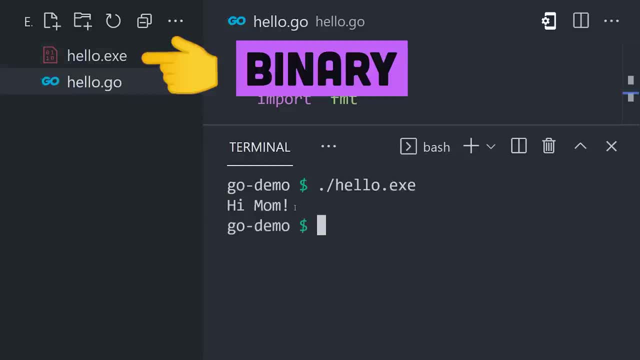 the source code and dependencies into an executable binary. When it comes to doing this, it's very easy to do. You just need to import the code and you'll be fine To create dependencies, we can also link to remote packages on GitHub Run go mod init. 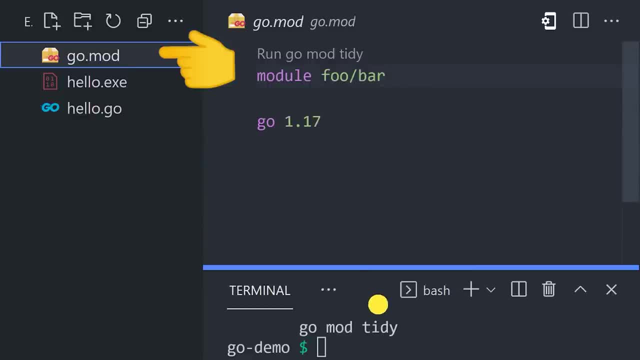 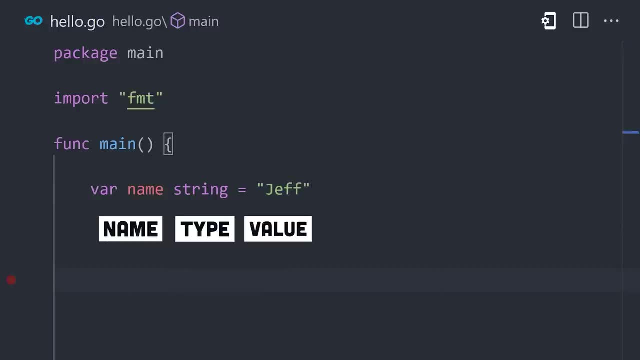 from the command line and that creates a go module file that enables dependency tracking. Syntactically, Go is like a concise version of C or C++. Declare a variable with the var keyword, followed by its name and type, and initialize it with a value. Or you might use 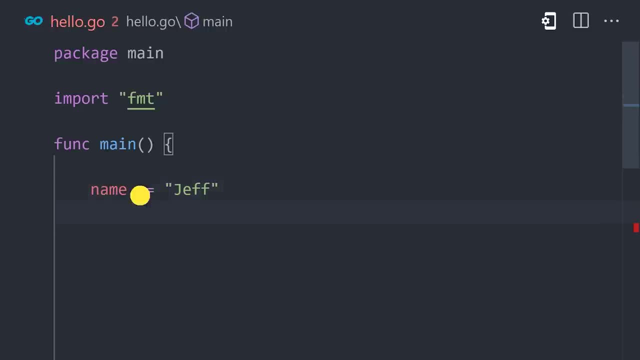 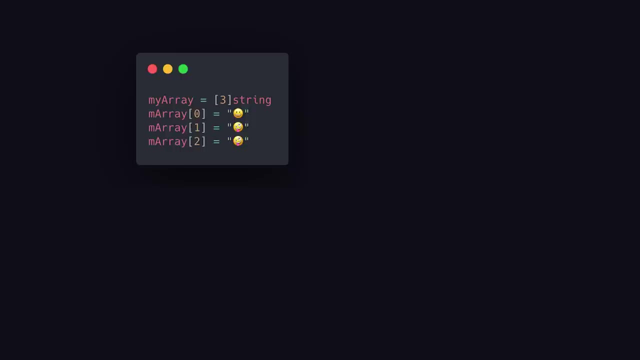 the short assignment syntax to replace var and let Go automatically infer the type, And you can define multiple variables from a single line. Go has all the other features you would expect in a programming language, like arrays, methods, maps, loops and control flow, but also allows you to store the memory address of a value. 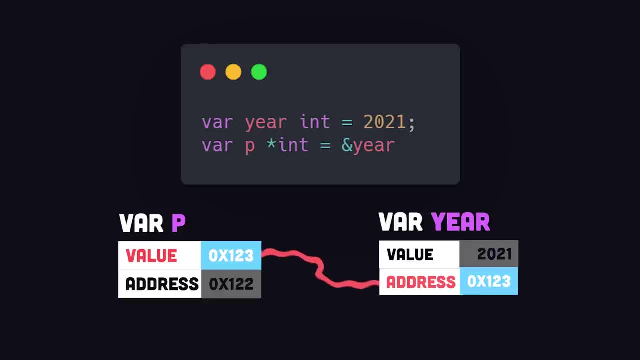 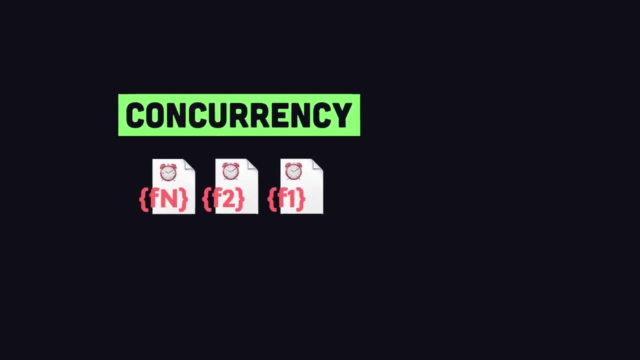 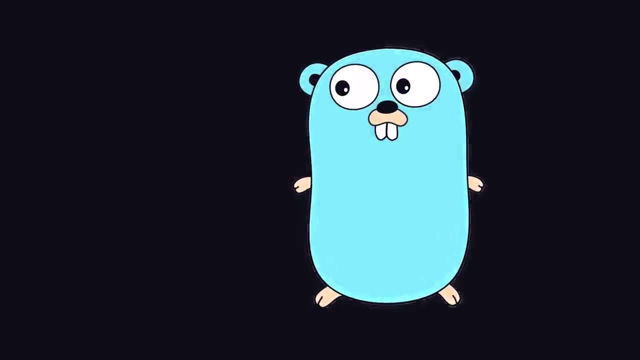 using pointers, while disallowing pointer arithmetic, which often leads to dangerous and unpredictable behavior. In addition, it supports concurrency with Go routines, which are functions that can run at the same time as other functions by utilizing multiple threads on a CPU. This has been Go in 100 seconds. Hit the like button if you want to see more short videos. 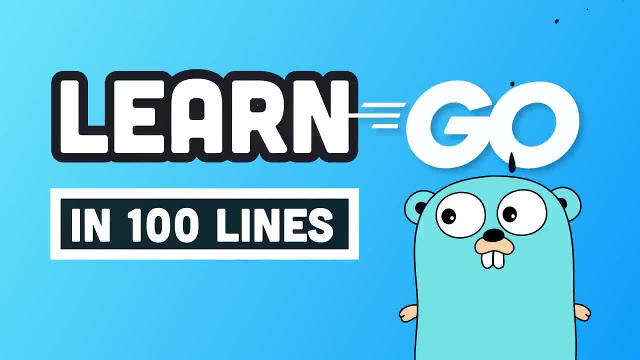 like this and check out the full article to write your first 100 lines of Go on, Fireship IO. Thanks for watching and I will see you in the next one.